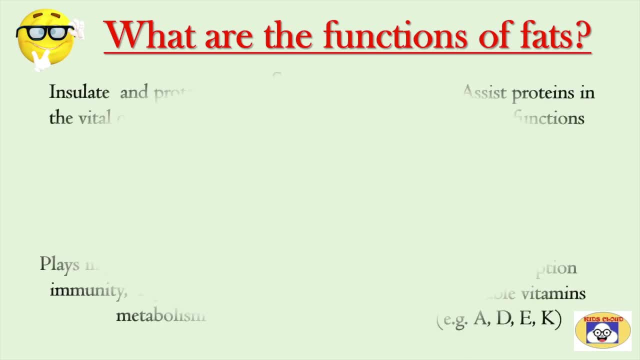 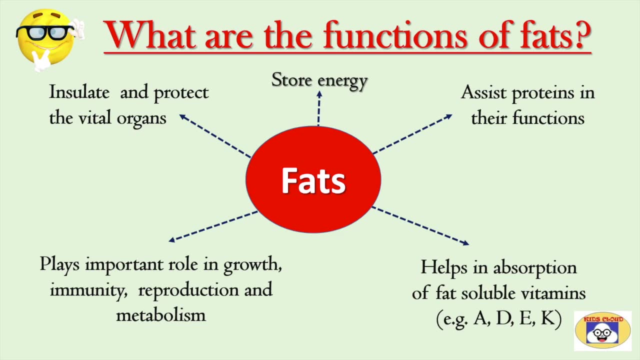 What are the functions of fats? Energy storage is the main function of fats. Besides, they assist proteins in their functions. Helps in absorption of fat-soluble vitamins- vitamin A, D, E and K. Plays important role in growth, immunity, reproduction and metabolism. Insulate. 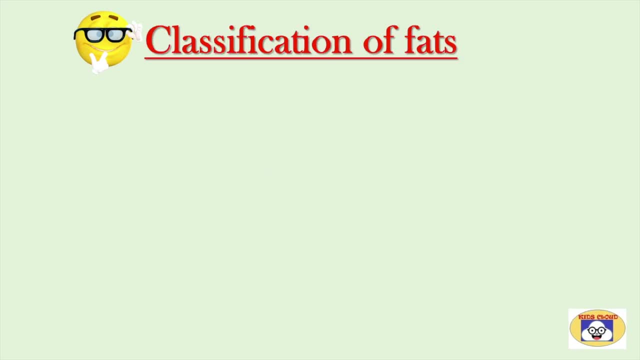 and protect the vital organs. Let's learn about classification of fats. Fats are classified into three main types: 1. Unsaturated fats. 2. Saturated fats. 3. Trans fats. Unsaturated fats are further divided into monounsaturated fats and polyunsaturated 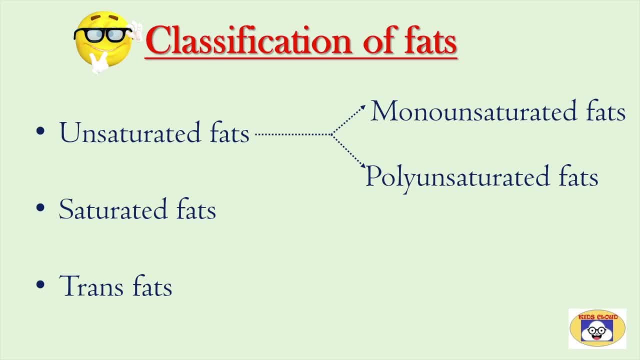 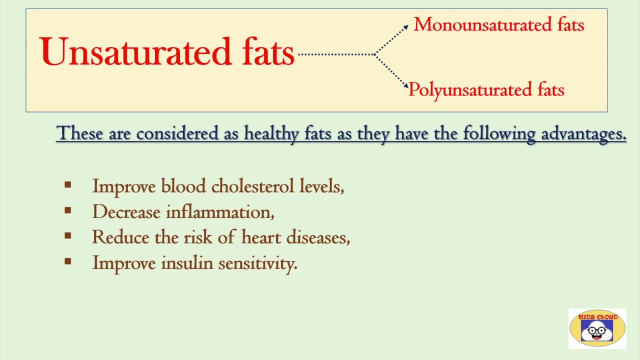 fats. In the next part of video, we will learn about food sources for these different types of fats. Unsaturated fats: These are considered as healthy fats as they have the following advantages: These fats: improve blood cholesterol levels, decrease inflammation, reduce the risk of. 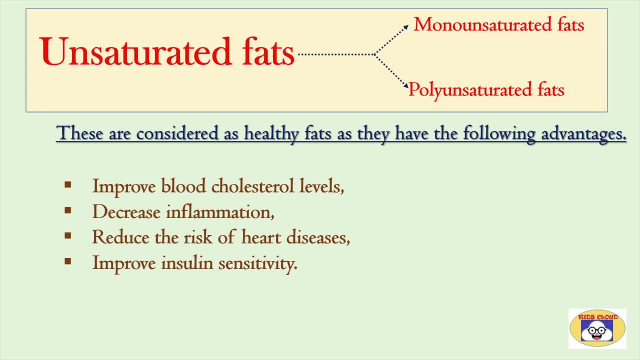 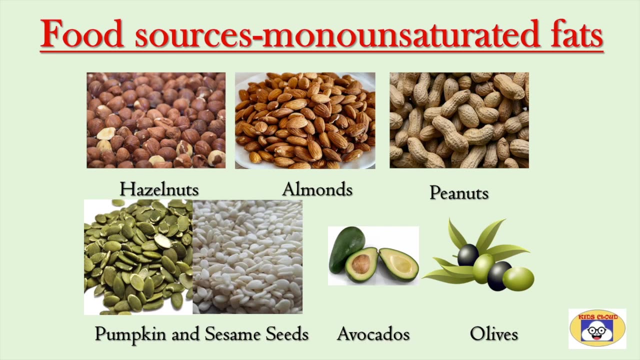 heart diseases improve insulin sensitivity. Vegetable oils, nuts and seeds are the main food sources for such types of fats. 1. Unsaturated fats: In following food sources we can get a good amount of monounsaturated fats. These mainly include hazelnuts, almonds, peanuts, pumpkin and sesame seeds, avocados and olives. Similarly, 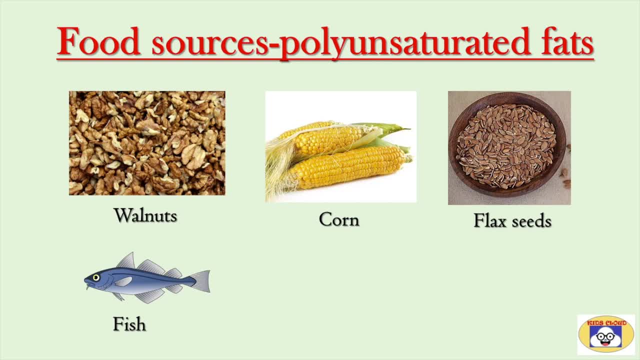 we can get polyunsaturated fats from walnuts, corn, flaxseeds and fish. Besides, polyunsaturated fats can also be used for other foods. 2. Polyunsaturated fats can also be used for other foods. These include nuts, walnuts. 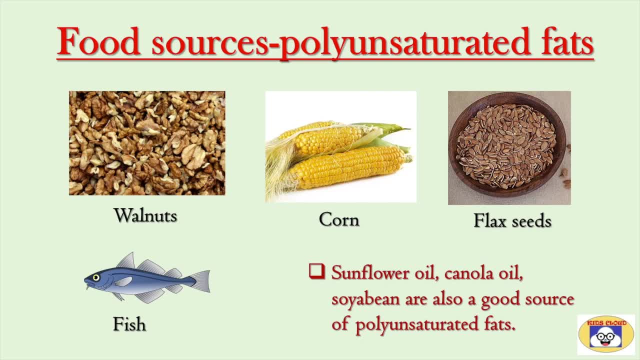 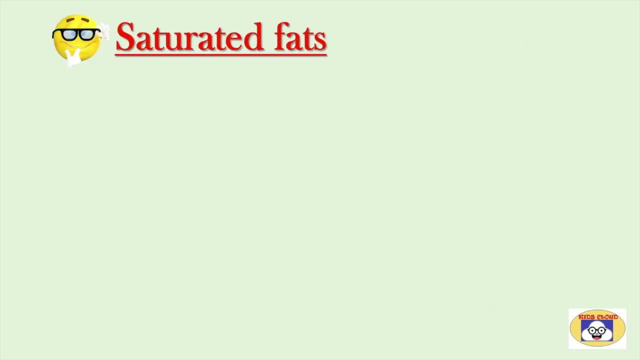 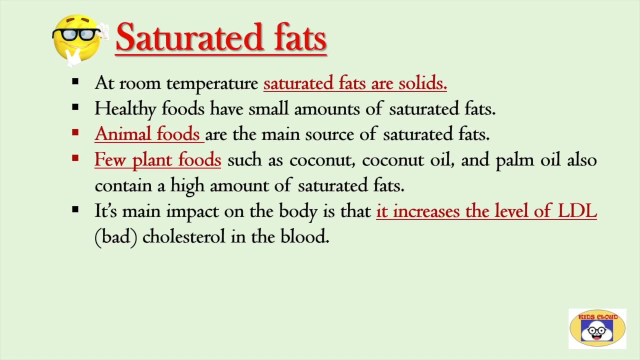 corn, flaxseeds and fish. 3. Sunflower oil, canola oil and soya beans are also a good source of polyunsaturated fats. 4. Saturated fats. At room temperature, saturated fats are solids. Healthy foods have small amounts of saturated 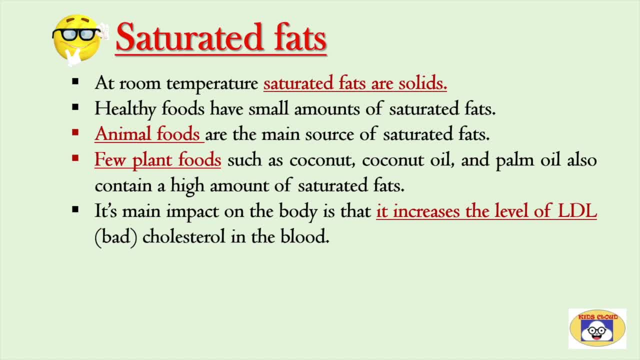 fats. Animal foods are the main source of saturated fats. Few of plant-based foods suggest saturated fats. foods such as coconut, coconut oil and palm oil also contain a high amount of saturated fats. Its main impact on the body is that it increases the level of LDL, ie bare cholesterol, in. 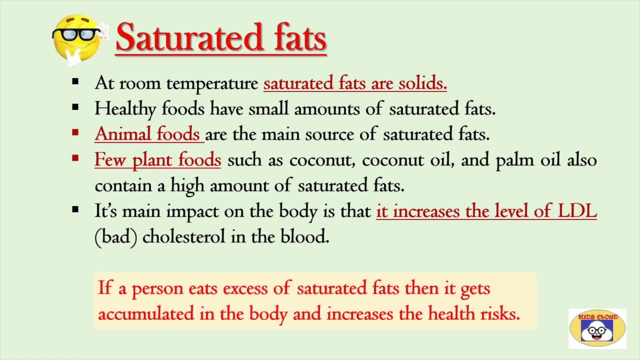 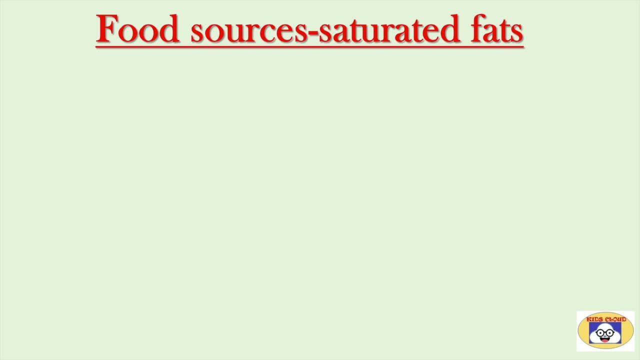 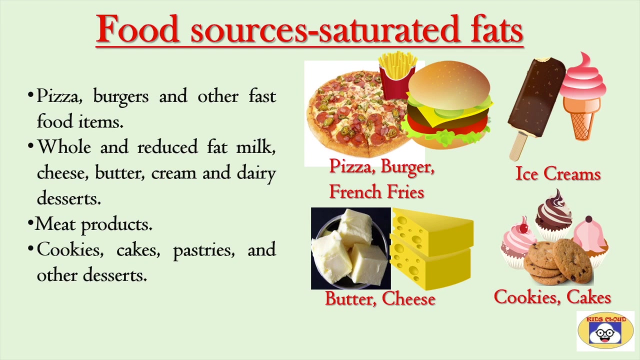 the blood. If a person eats excess of saturated fats then it gets accumulated in the body and increases the health risks. Most Sources of Saturated Fats- Mostly artificial food items which are flavored and tempting- give your body more saturated fats. These mainly include pizza, burgers and other fast food items. whole and reduced fat milk. 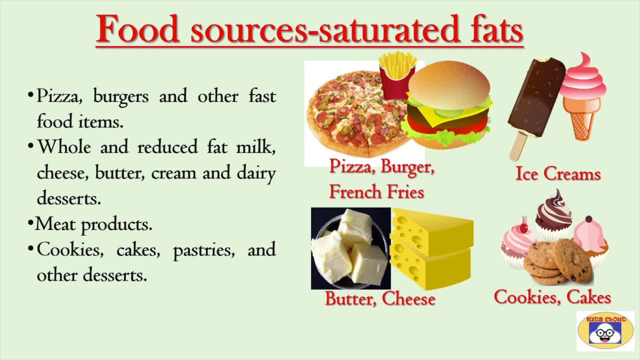 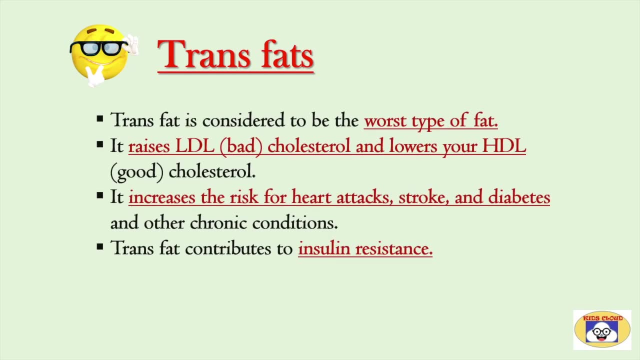 cheese, butter, cream and dairy desserts. Meat Products, Cookies, cakes, pastries and other desserts. Trans Fats: Trans fat is considered to be the worst type of fat. It raises LDL ie bad cholesterol- and lowers your HDL ie- good cholesterol. 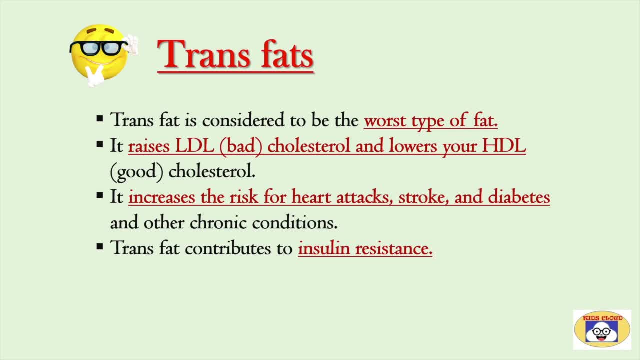 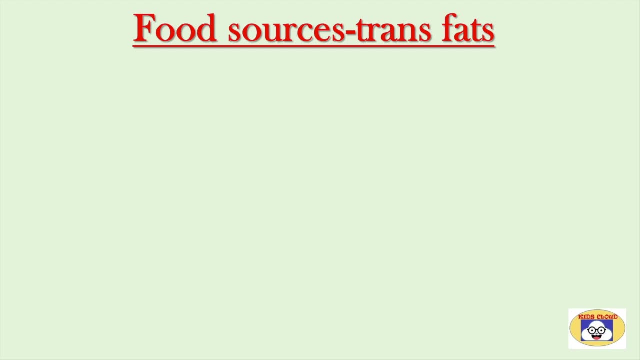 It increases the risk for heart attacks, stroke and diabetes and other chronic conditions. It also increases the risk of heart disease. Trans fat contributes to insulin resistance. Similar to saturated fats, trans fats are also found in most of the fast food items. These are some of the examples of food sources for trans fats. 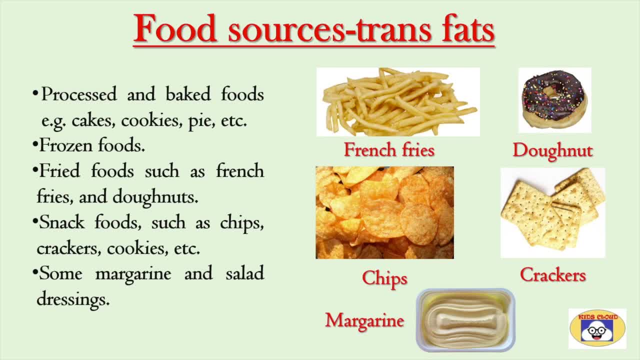 Processed and baked foods: ie cakes, cookies, pie, etc. Frozen foods, Fried foods, Snacks, Snacks, Snacks, fruits such as chips, crackers, cookies, etc. Some margarine and salad dressings also contain large amount of trans fats, which are not good.